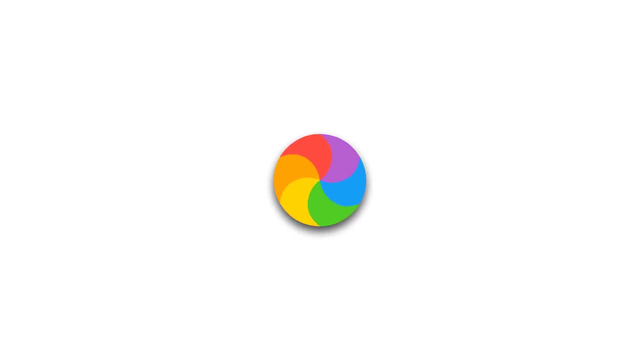 There it is: The spinning wheel of death caused by an infinite loop in a computer program. Wouldn't it be great if we had something that could find these infinite loops so that we could catch them? Let's be clear about what we mean. For example, the program. while true, 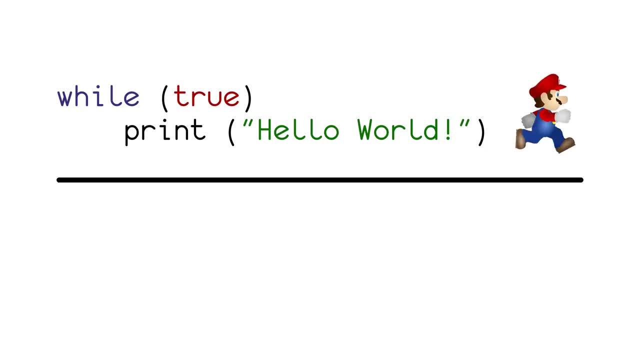 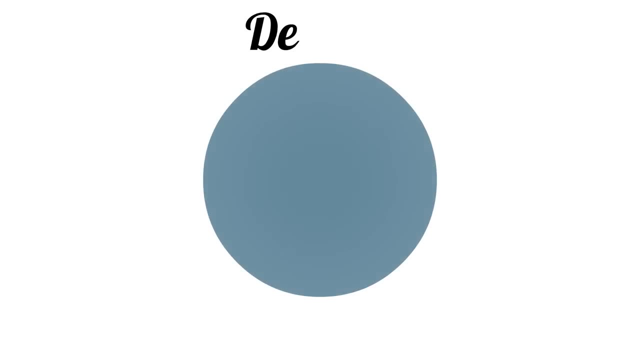 print hello world will loop forever, but the program that is just print hello world halts after printing hello world. What we want to do is create an algorithm, the decider, that takes in a program and an input for the program and can tell you if the program halts. 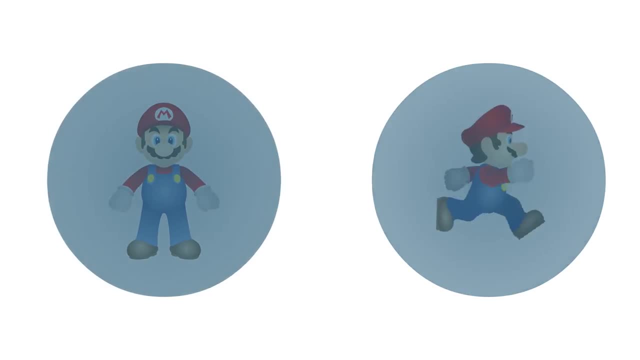 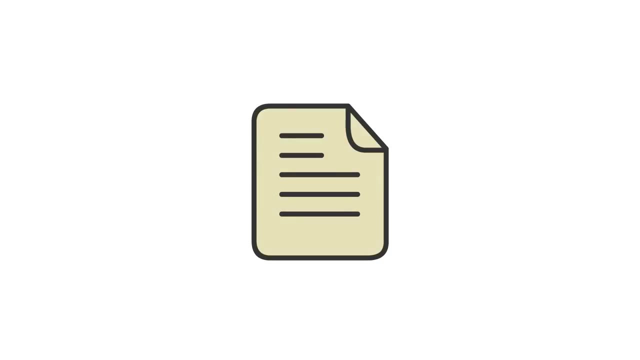 or loops forever when run on the input. It may seem a little weird to feed a program into another program, but to a computer a program is just a text file. As we'll see in a future video, this means that it's really just one big 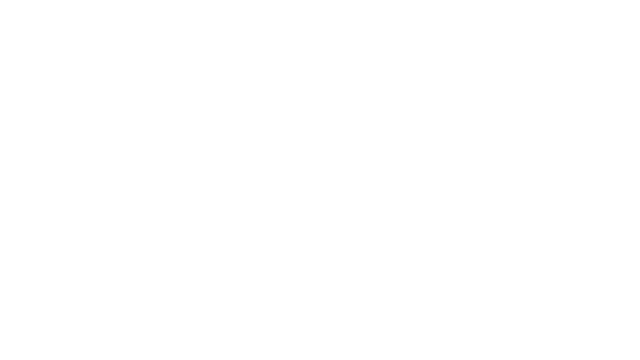 and giving a number to a program isn't really a big deal. Determining if a program loops or halts on an input is known as the halting problem and is extremely hard. In fact it's so hard that it's undecidable or impossible to solve. I want to emphasize that when I say 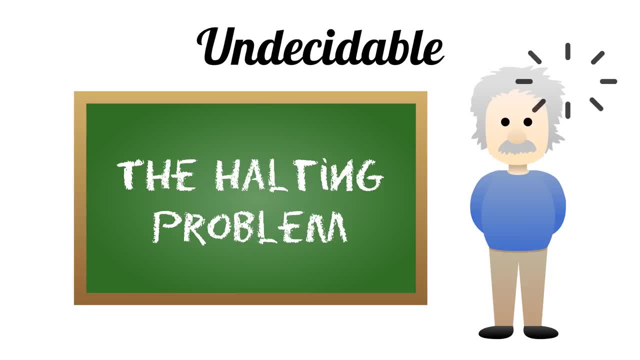 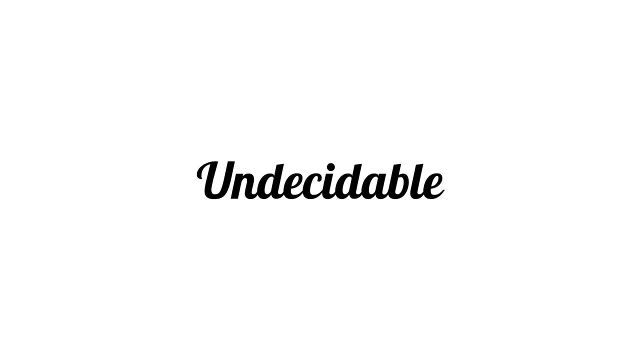 impossible. I don't mean that we're looking for a better solution or that we're trying to find an answer. I mean that, no matter what we try to do, we'll never come up with a program that can solve the halting problem. 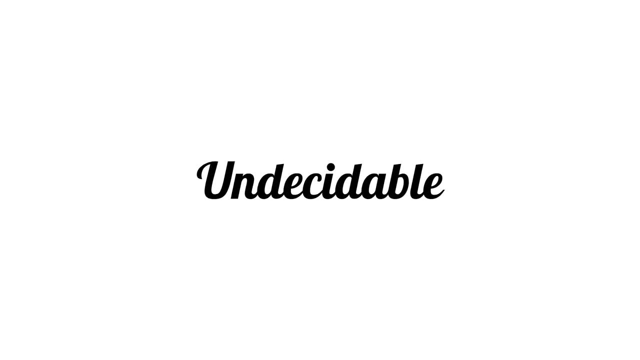 Let's think of a program that can solve the halting problem. Let's think of a naive algorithm or procedure to get an intuition as to what makes this problem so hard. For example, our solution might be always say it halts. Our solution could also be always. 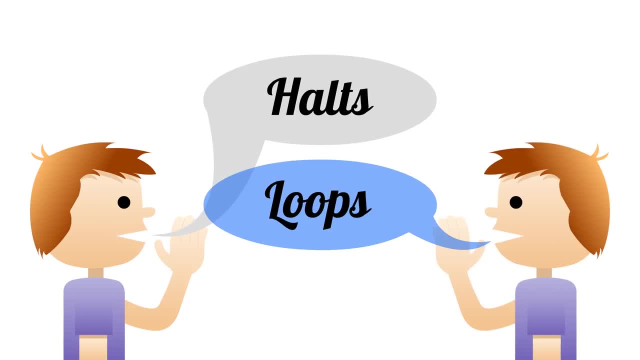 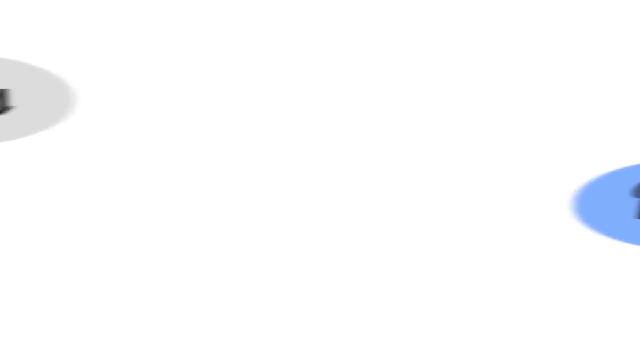 say it loops For any given program. one of these two solutions must be correct, but the other will also be wrong. Let's try making a program that won't give a wrong answer. Maybe our algorithm lets the program run on an input for a second and then we check if it halted or not. If it didn't, 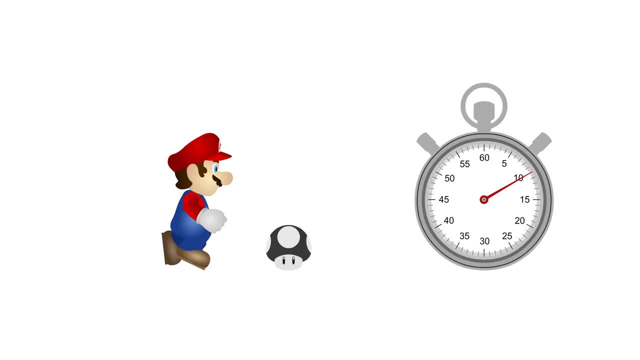 well, let's try making a program that won't give a wrong answer. Let's try making a program that won't give a wrong answer. Well, maybe it just needs 10 seconds. If it still didn't, well, maybe it just. 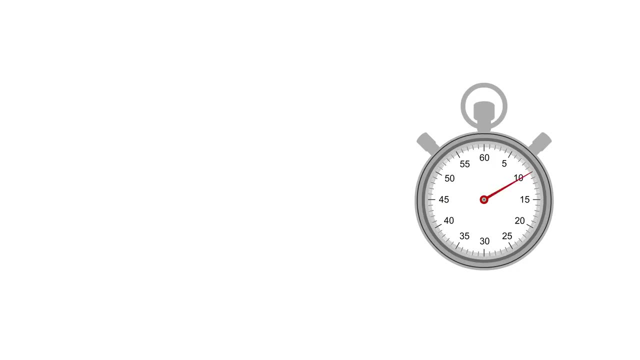 needs an hour. This quickly turns into a slippery slope where our decider just loops forever if the input program loops instead of giving an answer, Rather than solving the problem, we just reiterated it. In order to prove that the halting problem is undecidable, we'll use a technique called. 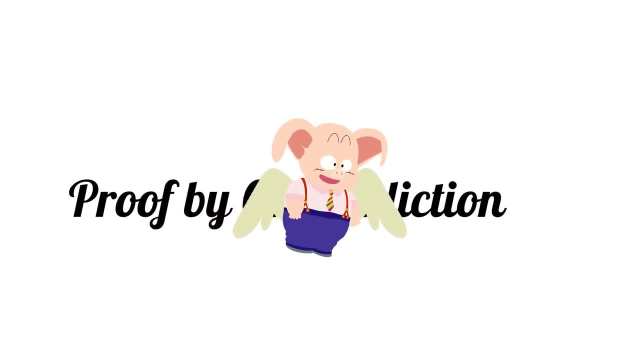 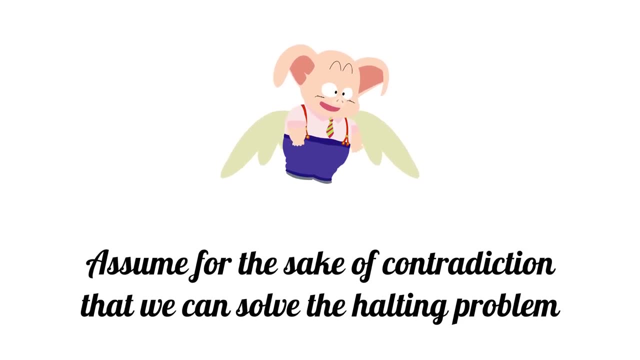 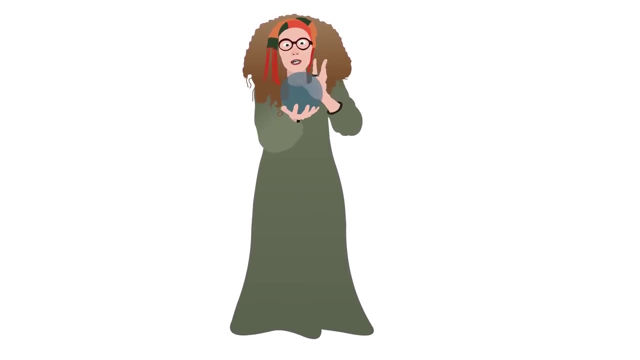 proof by contradiction. If you don't understand how it works, check out our previous video, where we proved that there are different sizes of infinities. So assume for this problem that the input is one big tree and that the algorithm will always be able to tell you whether a given 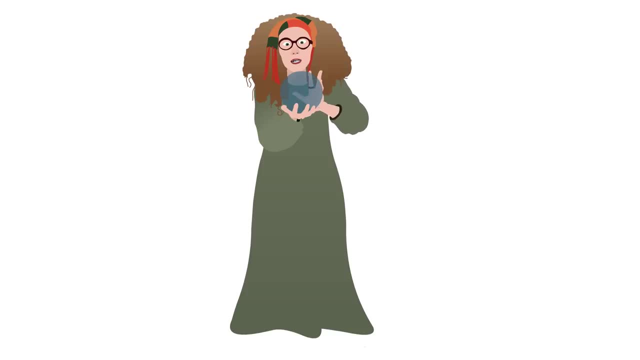 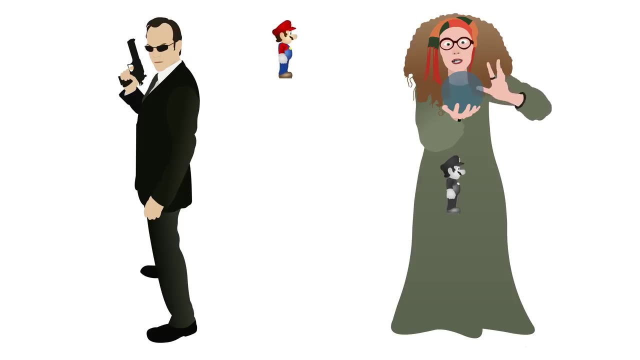 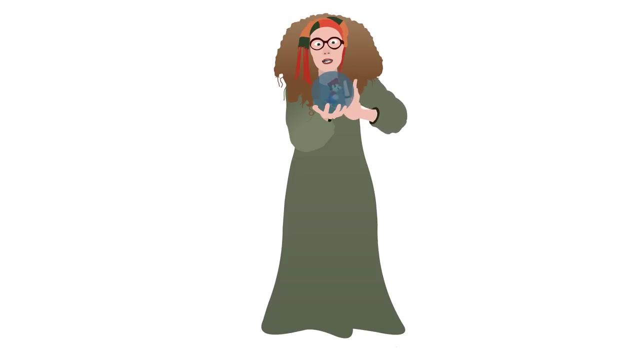 input is halted. What we're going to do is create a brand new program. let's call it Mr Smith. Mr Smith takes in a program as input and then asks the oracle what happens when that program is run with itself as input. If the oracle says that it loops forever, then Mr Smith will halt and 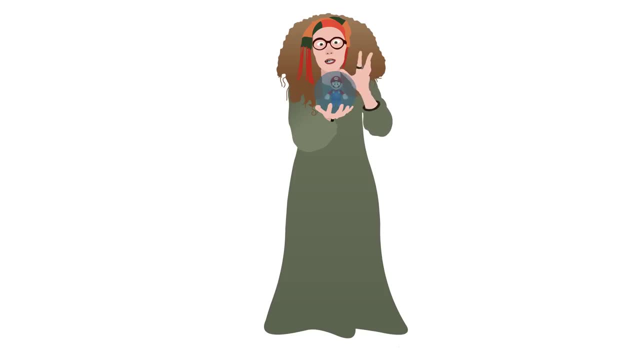 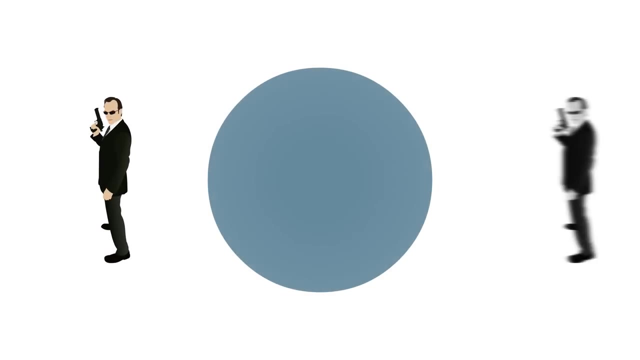 and call it a day. If the Oracle says that the program will halt, then MrSmith will loop forever. Now here's the interesting question: Does MrSmith, when given itself as input, loop or halt? Let's say that the Oracle predicts that MrSmith 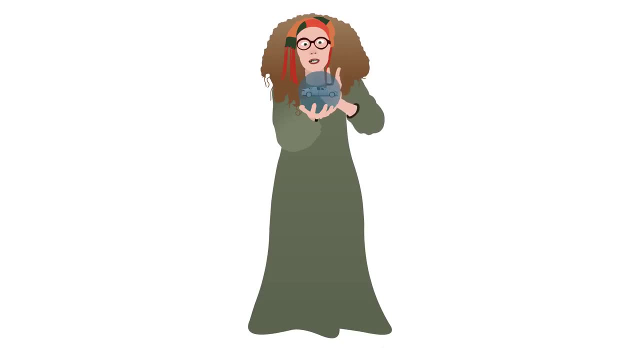 will loop forever when run on itself. But what does MrSmith actually do in that case? It halts. But if the Oracle predicts that MrSmith will halt, then MrSmith will actually loop forever, Like a rebellious teenager. MrSmith is 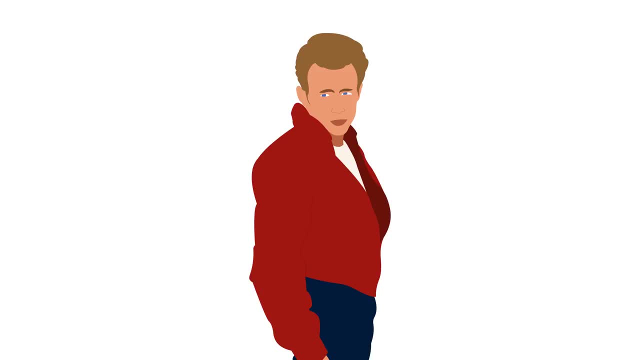 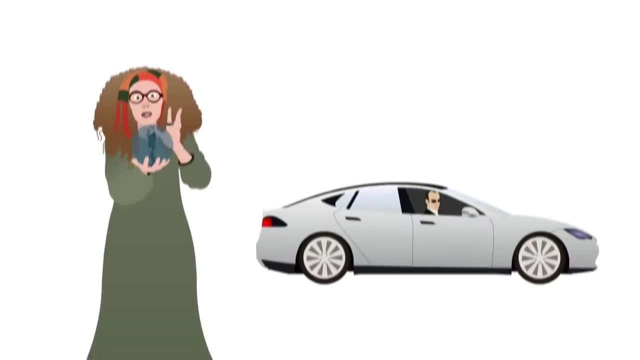 designed to do the opposite of whatever the Oracle says it should do. This means that whether MrSmith actually loops or halts, the Oracle must always give the wrong answer, Which means that the Oracle is a sham, contradicting our assumption that the Oracle solves the halting problem. All of these shenanigans with 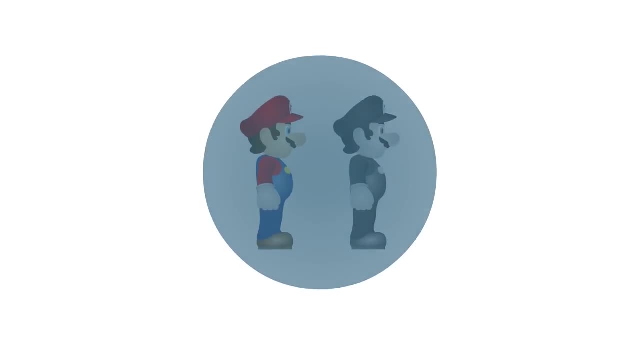 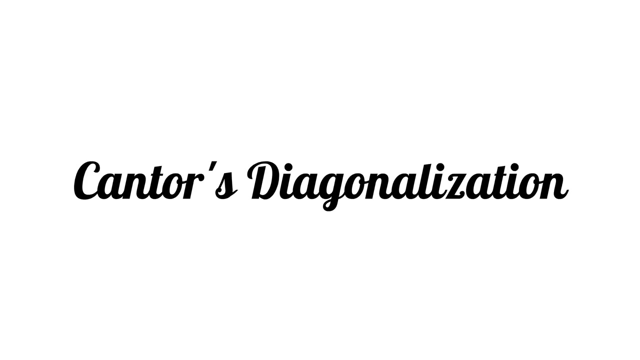 looping if it halts and halting if it loops, and programs getting fed into itself can all be very confusing. So let's think about this proof in understanding the problem. Let's look at it in another way, using Cantor's diagonalization. Be sure to check out. 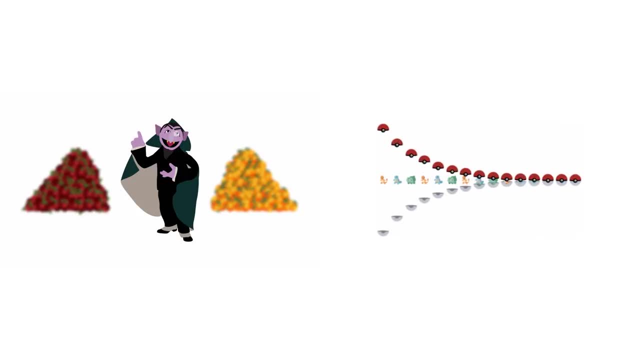 our previous videos on comparing infinities and Cantor's diagonalization. for a better understanding of this alternate proof, We'll start our new explanation the same way. Assume, for the sake of contradiction, that there exists an Oracle that solves the halting problem, As stated before: computer. 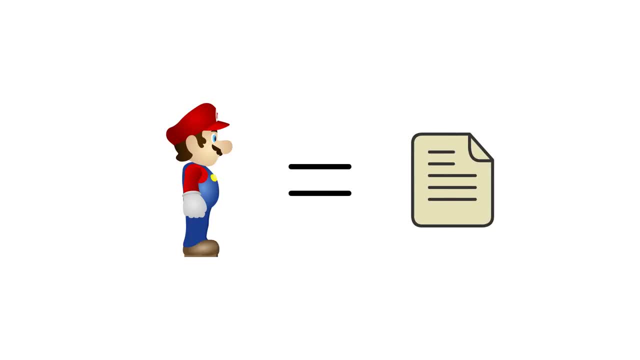 programs are really one big number, which means that the amount of all programs is countably infinite, So we can list out all of the possible programs. We can then create a grid by using all the possible input programs. Each program, when run on each input, will either loop or halt. 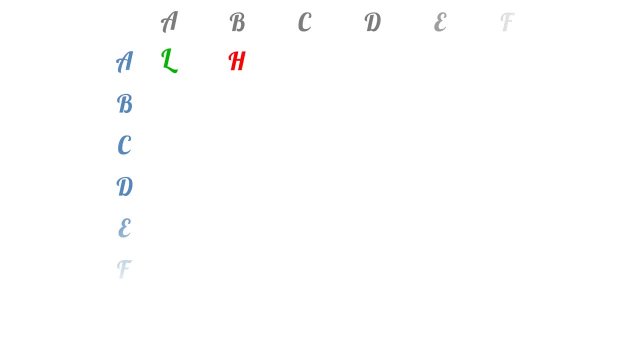 For example, maybe program A loops when run on A, halts when run on B, loops when run on C, etc. Maybe program B halts on all inputs. Let's take this list as an example of what each program might do when run on each input. Now we create a new row by taking each element. 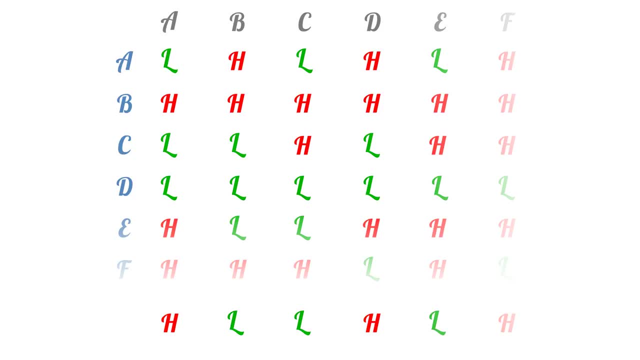 off the diagonal and flipping halt to loop and loop to halt. Where does this new row appear on the list? By the diagonal argument, it can't appear anywhere on this list since it's different from every row in at least one place. Since the list is a complete list of all computer programs, that means that 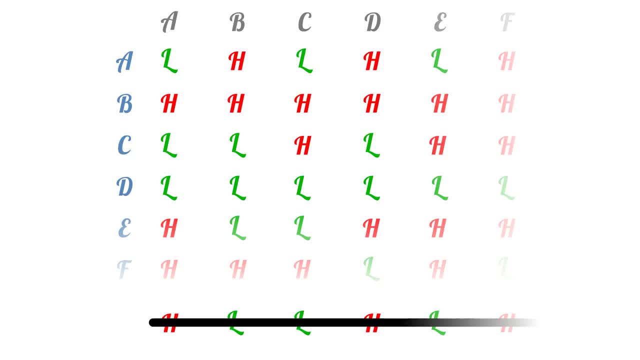 we can never write a program that matches the new row that we generated on all inputs. However, if we had the magical oracle that could solve the halting problem, it would be pretty easy to make the program that matches this row. In fact, that's what we did with Mr Smith. If you notice what Mr Smith does it. 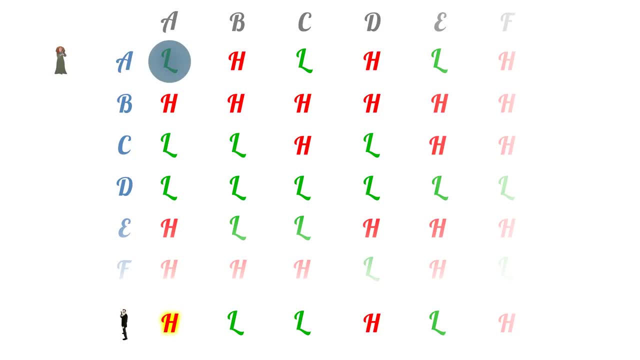 looks at what A does when run on itself, and then does the opposite. The same for B, C and every other program that we could write. Since we know that Mr Smith can't actually exist, it must mean that the magical oracle also can't exist. The. 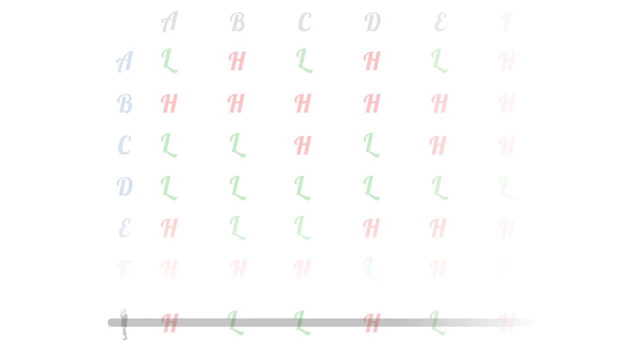 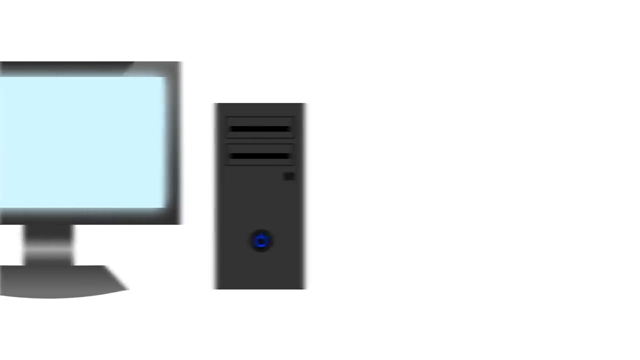 undecidability of the halting problem is interesting in and of itself, but was also integral to the history and development of computation, as well as the nature of computation. This proof first appeared in Alan Turing's landmark paper on computable numbers with an application to the 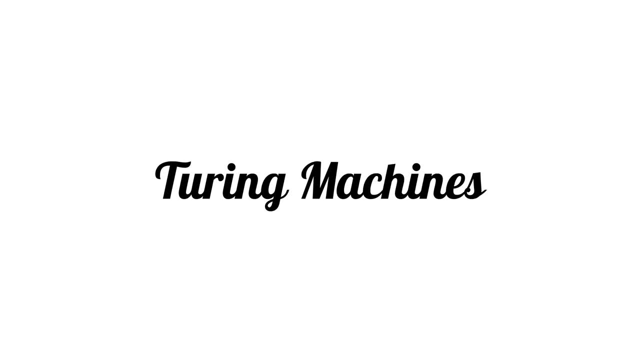 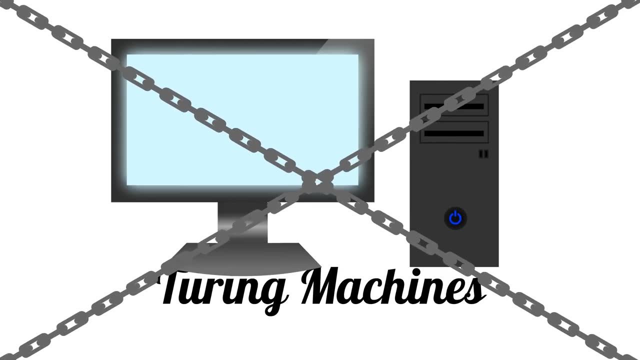 Eng-Scheidung's problem, where he created Turing machines, which form the basis of what computers are today. These undecidable problems may show fundamental limitations in computation, but Turing also demonstrated the universality of his machines in the appendix of the same paper. 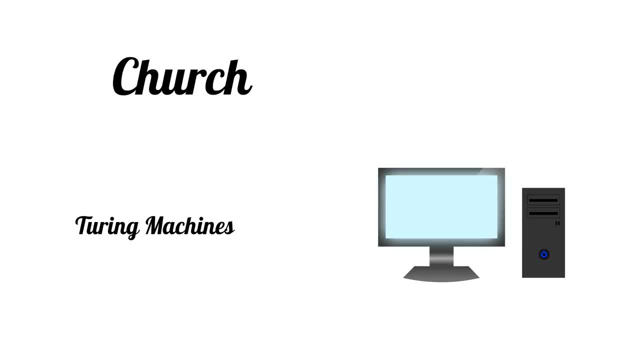 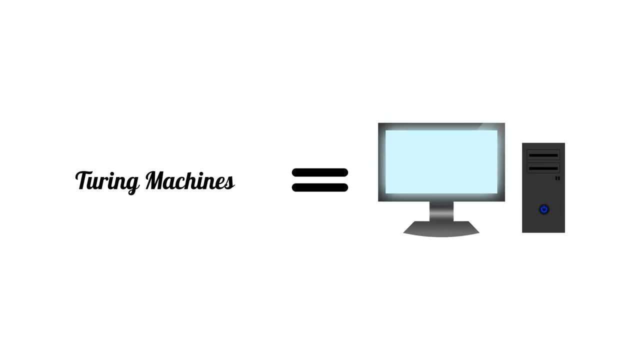 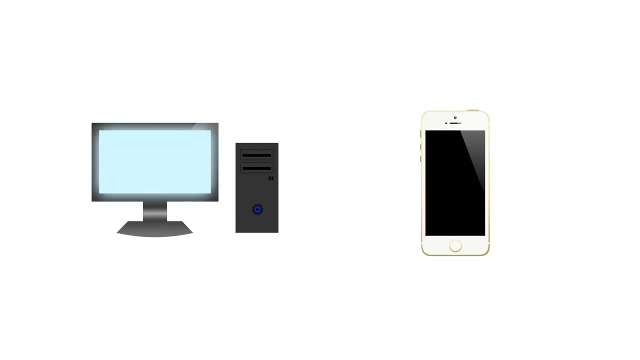 That work continued into what is now called the Church-Turing thesis, which says that all models of computation are the same as Turing machines. If you had any doubt as to how powerful Turing machines really can be, just take a good look forward, or in your pocket, Computers may not be able to solve the 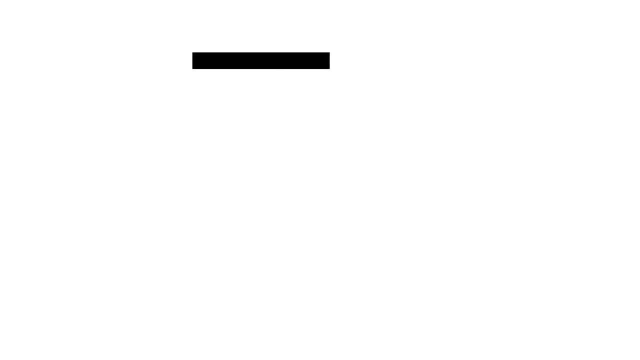 halting problem, but they sure can do a lot.